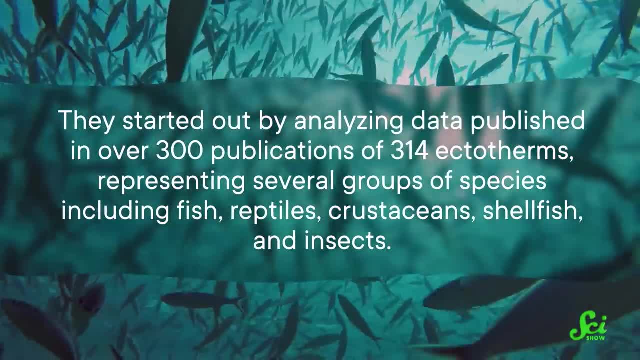 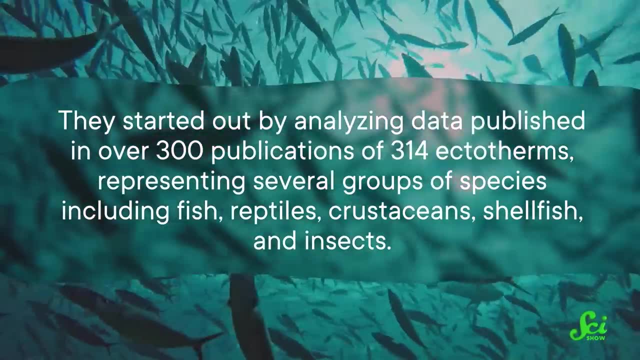 They started out by analyzing data published in over 300 publications of 314 ectotherms representing several groups of species Including fish, reptiles, crustaceans, shellfish and insects. They looked at everything from these creatures' heart rates to how fast they move to their 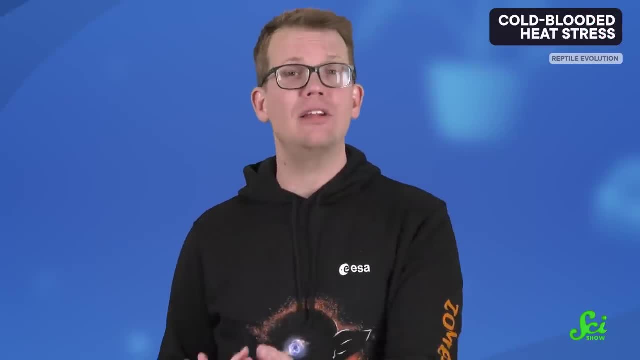 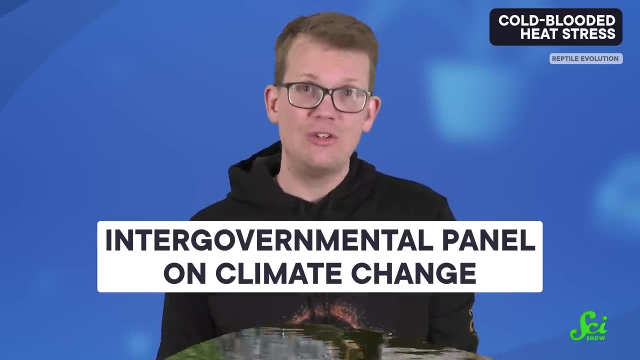 metabolisms, And what they found was that even the more modest increases in global temperature, as predicted by the Intergovernmental Panel on Climate Change, will be extremely stressful for these creatures. They dug further into the data by reviewing over 120 published studies on heat failure. 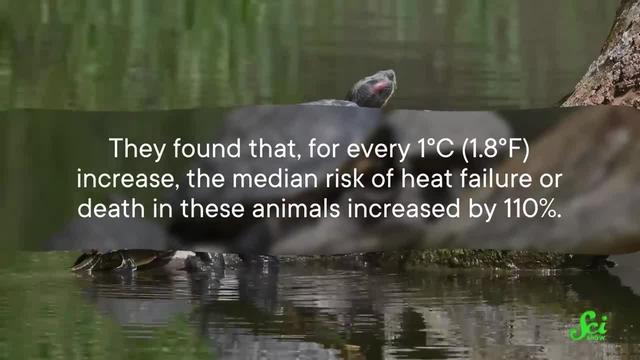 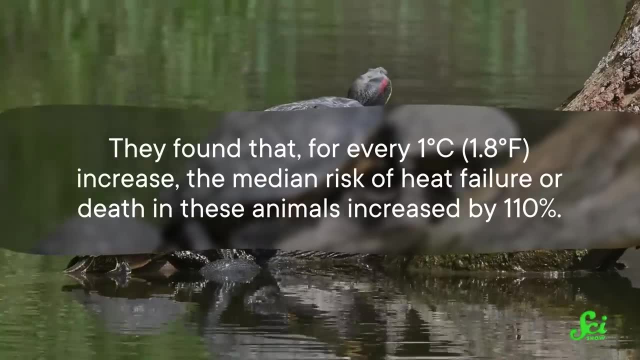 for 112 ectothermic species. They found that for every one degree Celsius increase, the median risk of heat failure or death in these animals increased by 110 percent. As the climate changes, more ectotherms will be exposed to the upper limits of their temperature. 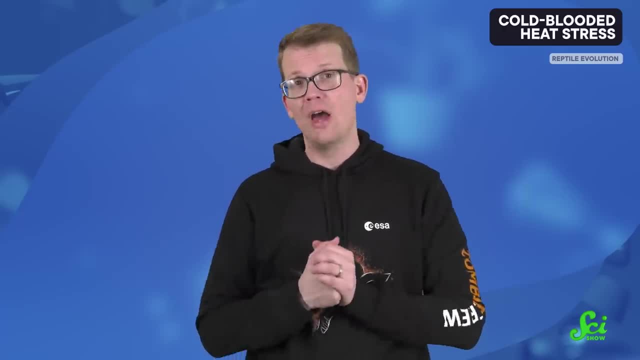 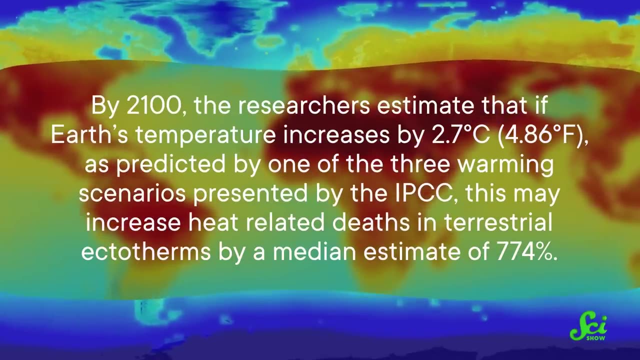 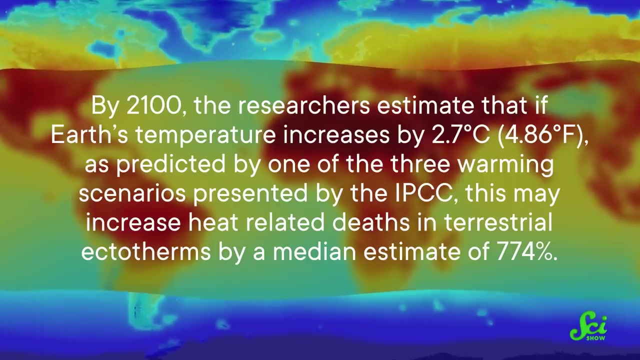 thresholds for longer periods of time, Because those temperatures will become the new normal, not just a short swing into the danger zone, By 2100,. the researchers estimate that if Earth's temperature increases by 2.7 degrees Celsius, as predicted by one of the three warming scenarios presented by the IPCC, this 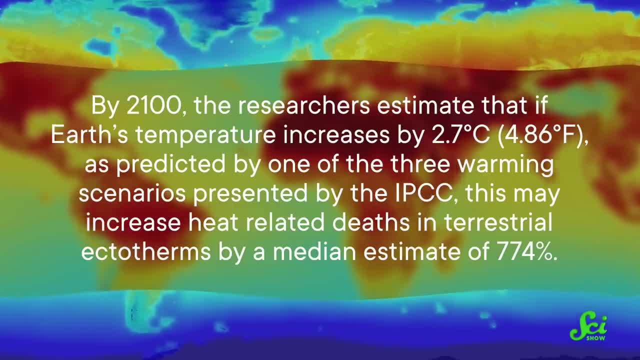 may increase heat-related deaths in terrestrial ectotherms by a maximum. That's what they're trying to do. They're trying to increase heat-related deaths in terrestrial ectotherms by a maximum, And they're doing it with a median estimate of 774 percent. 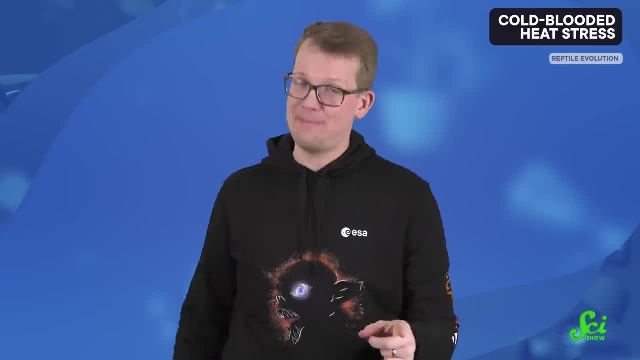 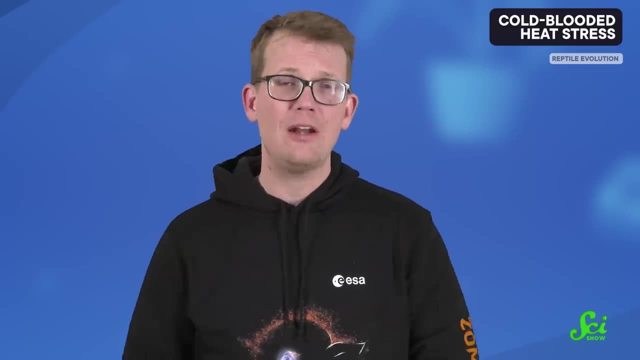 For aquatic ectotherms the estimate is only 180 percent, And even in the more modest suggested temperature increase of just under 2 degrees Celsius, which is pretty much locked in at this point, the impact of these temperature changes on ectotherms is going to be much more significant than previously expected. 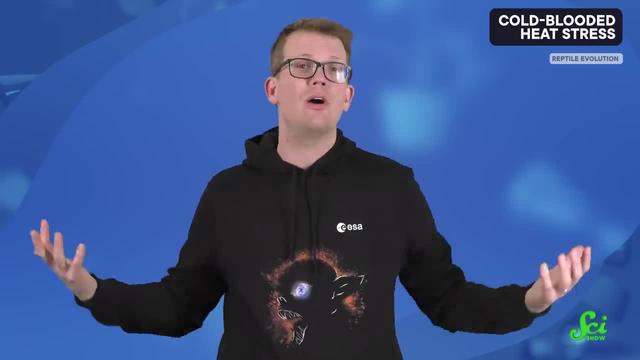 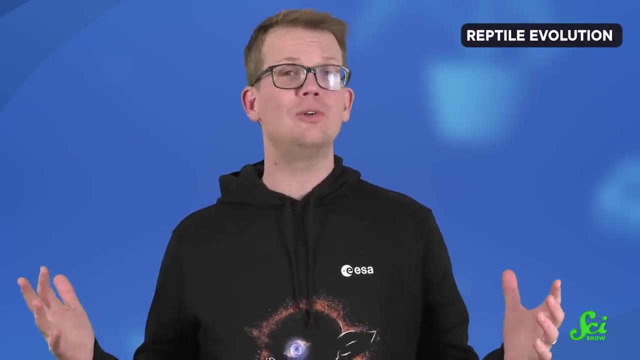 Which matters, because species don't exist in a vacuum. They are part of complex food webs and we're going to have to account for their absence in future climate scenarios. Speaking of cold-blooded creatures… When we picture the Jurassic period, we'd generally imagine dinosaurs. 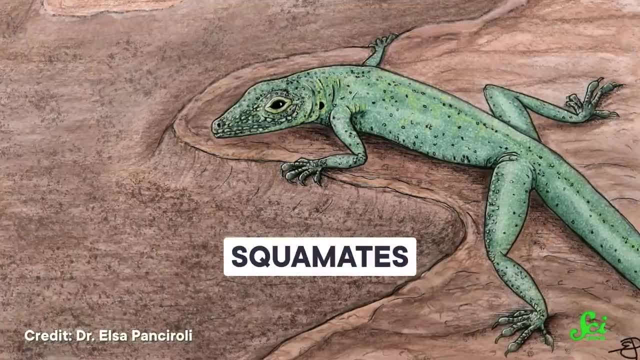 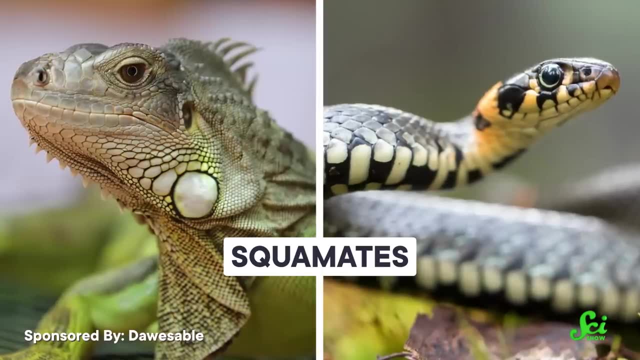 But another paper published in Nature This Week describes an early relative of squamates. Squamates are a diverse group of scaled reptiles that today makes up more than 10,000 living species, ranging from snakes to lizards. All squamates descended from a common ancestor who lived around 240 million years ago during. 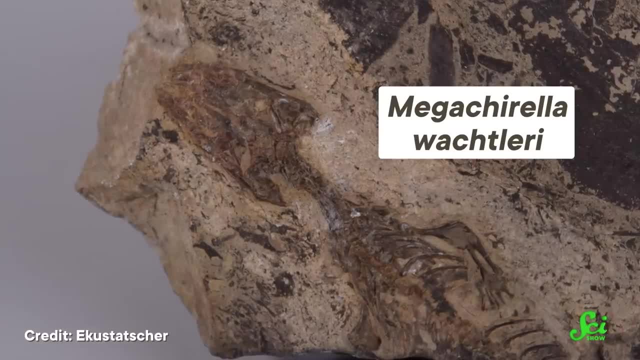 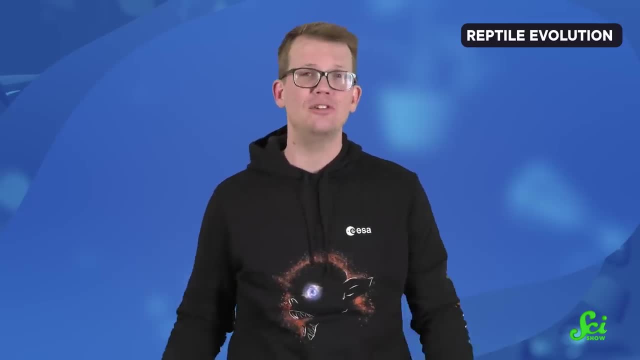 an era that was ruled by dinosaurs. That common ancestor would have contributed many features to squamates that we know today, But the fossil record is pretty incomplete. It's hard to believe. There's a lot of uncertainty around the evolution of their anatomy and which species 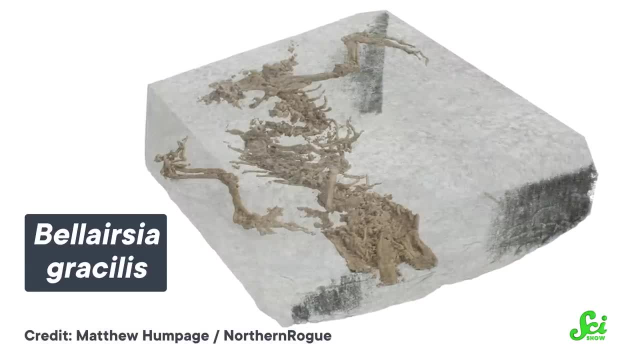 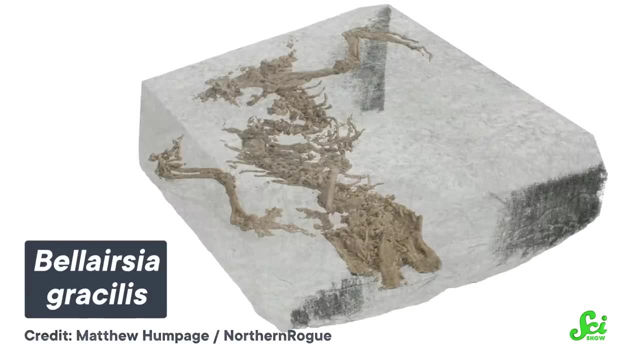 diverged when. But this well-preserved fossil discovered in Scotland can help fill in some of the gaps surrounding the evolution of the squamate body plan and where they lived on Earth during the Jurassic era. In the new study, researchers were able to take a look at which traits were ancestral. 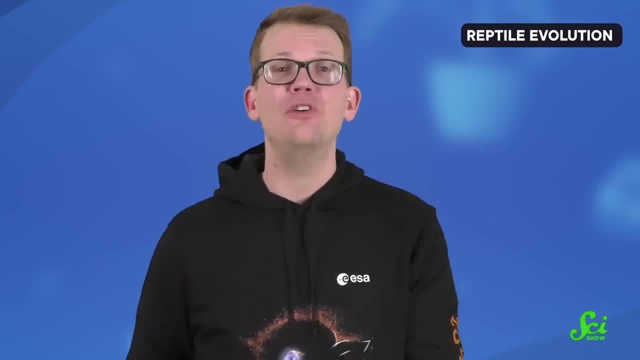 or inherited from the common ancestor of all squamates. That helps us understand what hand every creature in the group has been dealt. In the case of this creature, the roof of its body is the same as the roof of its body. In the case of this creature, the roof of its body is the same as the roof of its body. 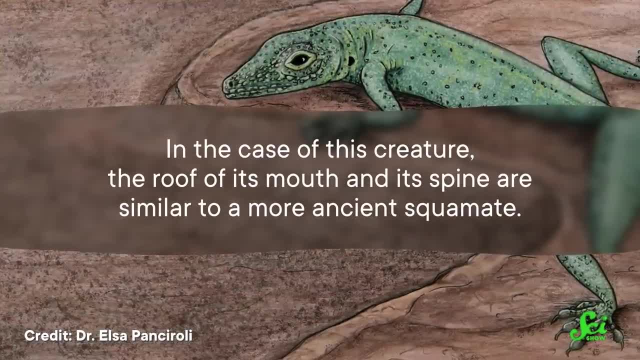 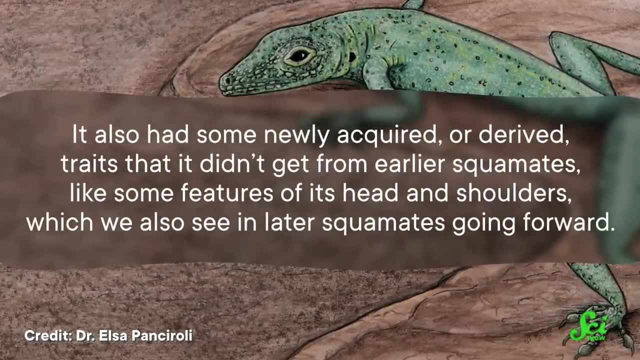 Its mouth and its spine are similar to a more ancient squamate. It also had some newly acquired or derived traits that it did not get from earlier squamates, like some features of its head and shoulders, which we also see in later squamates going. 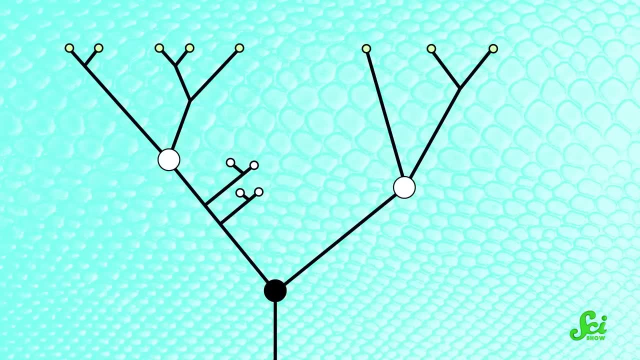 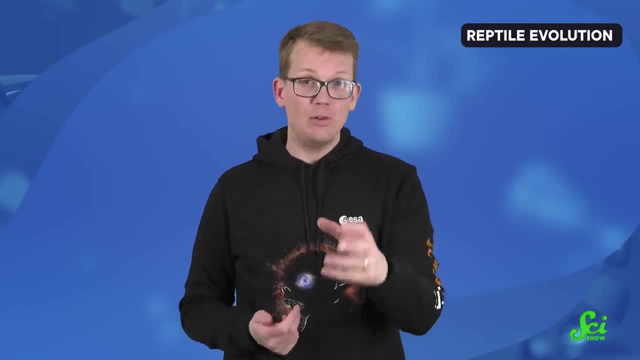 forward. Researchers believe that this particular species is a stem squamate, meaning an early branch near the base of the snake and lizard family tree. Its body plan sheds some light onto the evolution of squamates that we are familiar with, like the way that their skull bones move in relation to their jaws. 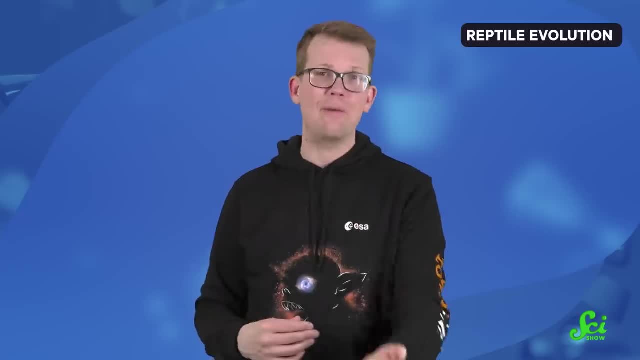 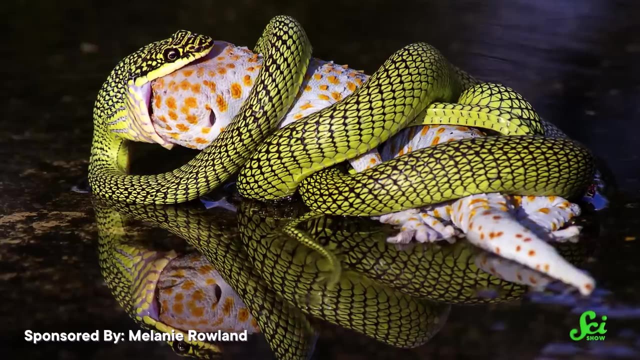 And, of course, the way that their legs move. Think about a snake opening its mouth way too wide to swallow prey, for instance. That's more in the skull than in the jaw, And this fossil's skull can tell us a bit about how features like that got started. 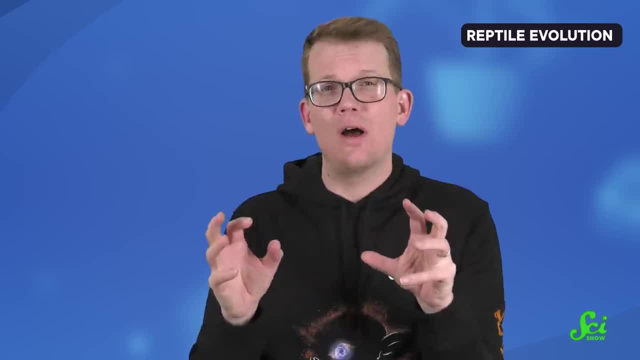 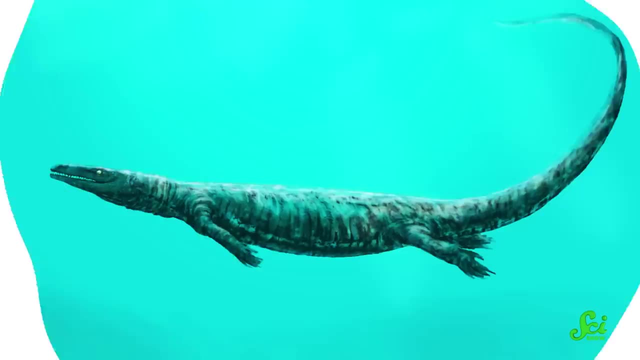 Also, this fossil may help untangle a little of the confusion surrounding squamates. because of the diverse amount of creatures that fall into the squamate category — everything from snakes to chameleons, to geckos, to extinct marine lizards- There's a lot of debate about whether certain groups like iguanas come earlier in that. 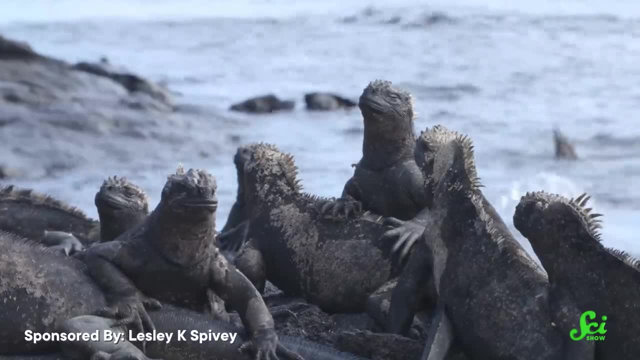 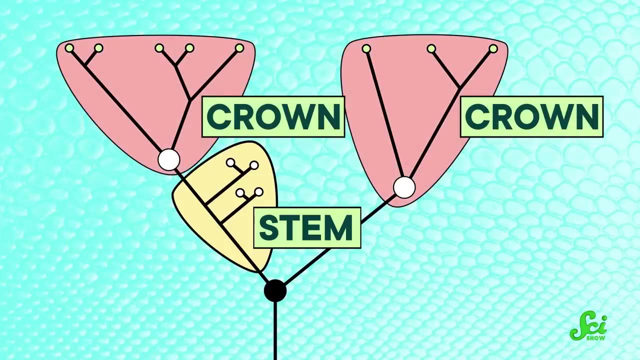 family tree or are more derived. This new fossil's body features may help resolve some of that ambiguity. Not only that, the researchers believe that it was coexisting with crown squamates, or ancestors of species that are still alive today, potentially hanging around them until